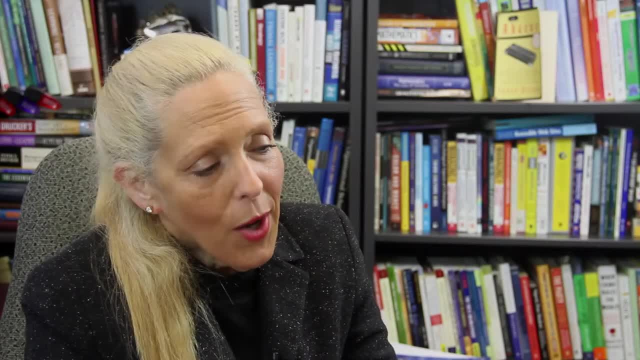 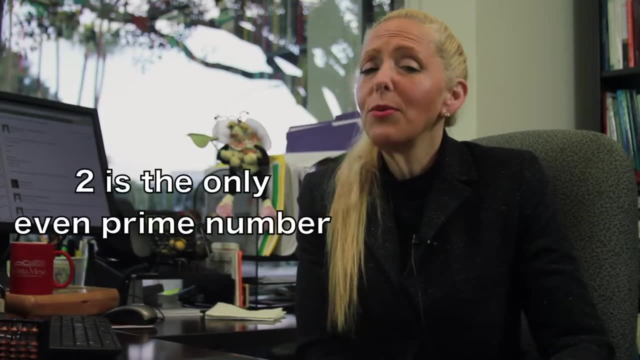 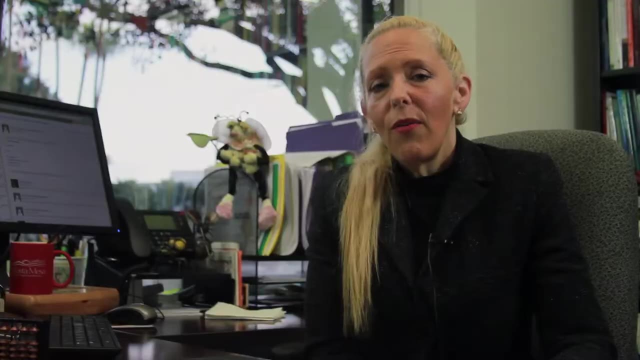 We will walk through these. First, 1 is not prime. Next, the first natural number that is prime is 2, and 2 is the only even prime number. 3 is only divisible by 1 and itself, so 3 is prime. 4 is a composite number because its factors are 1,, 2 and 4.. 5 is prime because its only factors are 1 and 5.. 6 is a composite number. 6 is a composite number because its factors are 1,, 2, and 4.. 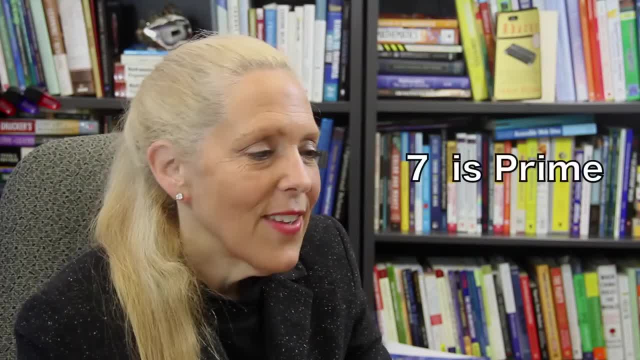 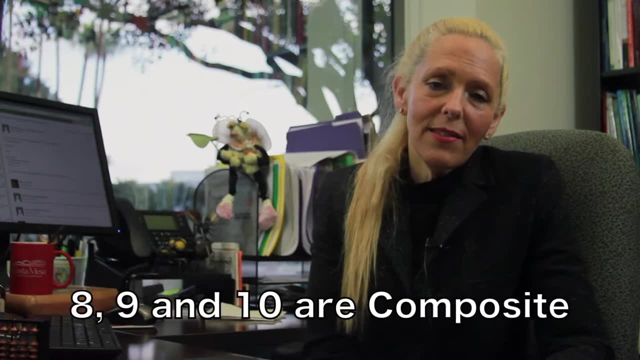 6 is a composite number because its factors are 1,, 2, and 5.. factors of six are one, two, three and six. Seven is prime because seven can only be broken down into the factors one and seven. Eight, nine and ten are composite. The next prime. 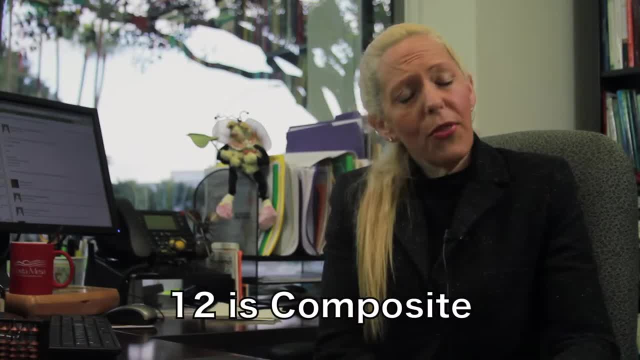 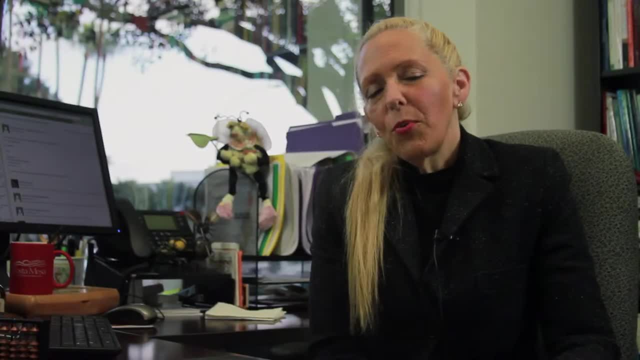 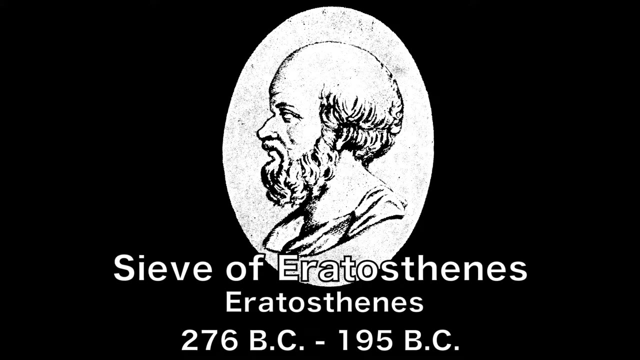 number is eleven. Twelve is a composite number, but thirteen cannot be broken down further, so it is a prime number. Long ago, the Greek mathematician Aristosthenes devised a technique called the sieve of Aristosthenes. He created a grid of a hundred numbers and showed how. to sift through the numbers. eliminate the composite numbers and leave only the prime numbers. Let's start with one. but one is not prime. One is not a composite number either. Put an x and the number one. The first natural number that is prime is two. Recall that two. 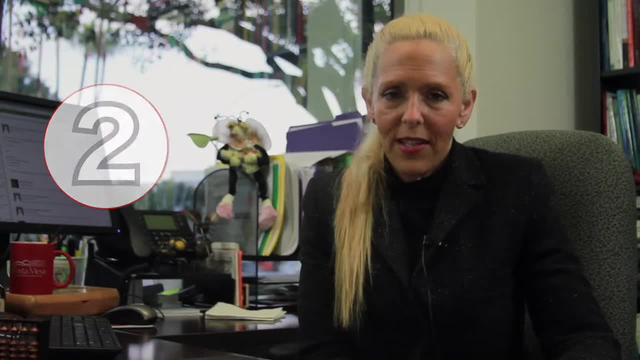 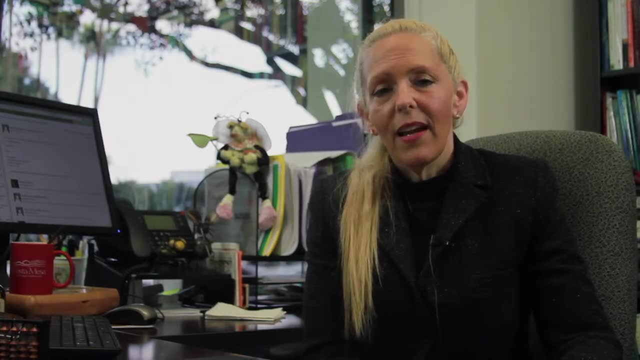 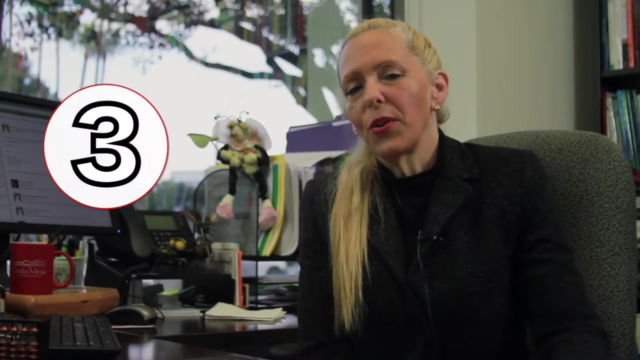 is the only even prime number. Put a circle around two. Since all of the multiples of two are composite numbers, shade those numbers. Now, three can only be broken down into the factors one and three. Thus three is prime. Put a circle. 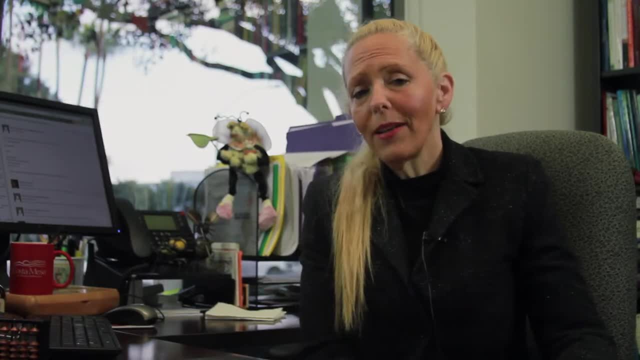 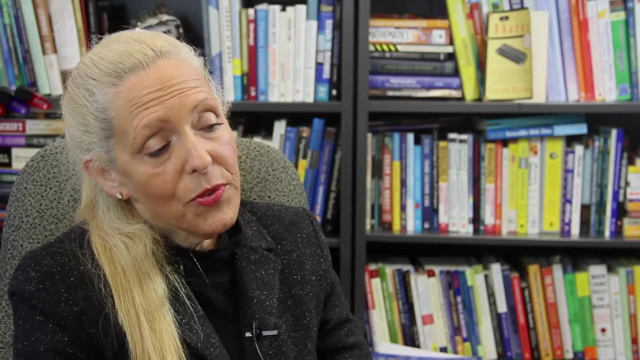 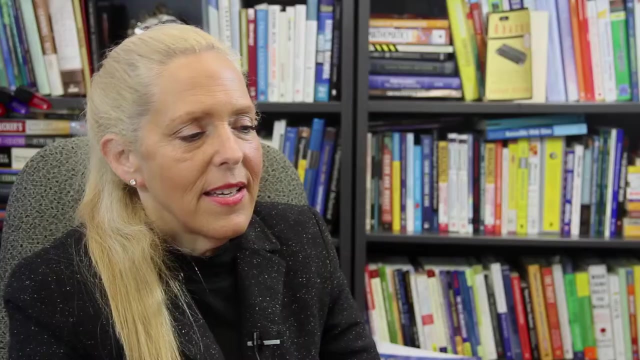 around three, But all of the other multiples of three are composite numbers, so include those numbers in the shaded region. Five is prime, However the multiples of five are composite numbers, So we circle the five and shade all of them. Seven is prime, so it is circled, but the multiples of seven are composite numbers. 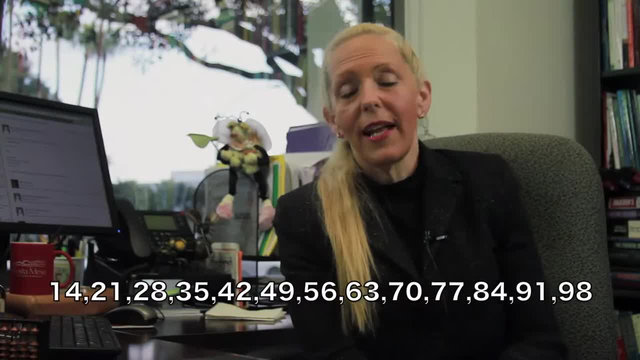 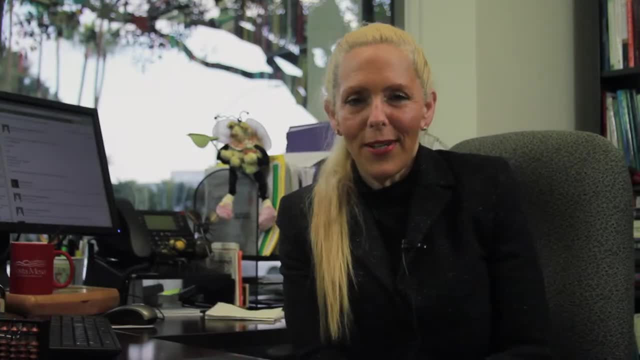 That means that 14,, 21,, 28,, 35,, 42,, 49,, 56,, 63,, 70,, 77,, 84,, 91, 98 are composite and they must be in the shaded region. Check the numbers left over that are not shaded: These: 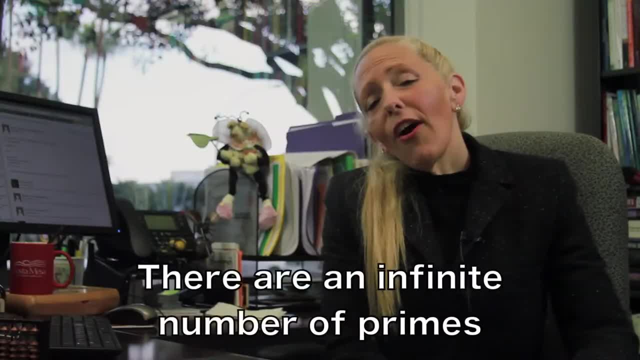 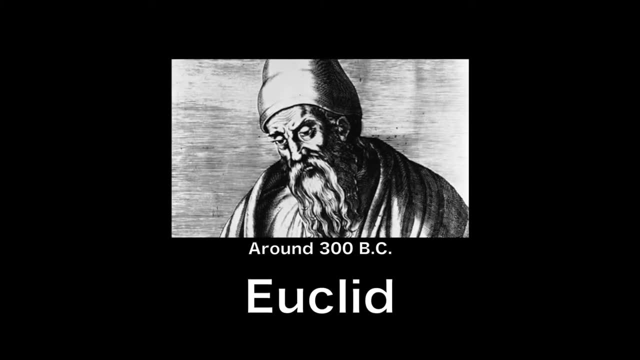 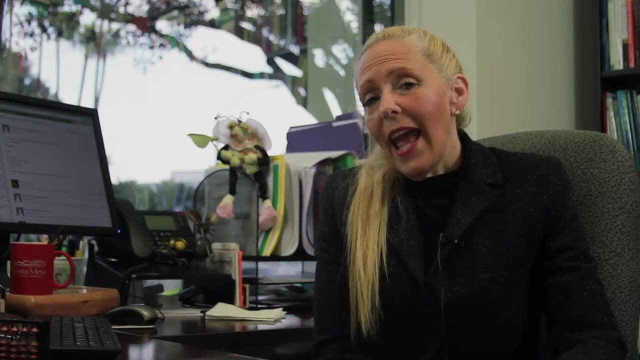 are all prime numbers. There are actually an infinite number of primes. This was proved by Euclid more than 2,000 years ago. A 17th century French monk named Marin Mersenne proved that any number in the form two to a prime number minus one is prime. Thus, since there, are an infinite number of prime numbers, then there should also be an infinite number of Mersenne primes, But each one must be painstakingly proven to be prime rather than determined by assumption. The first four prime numbers are two to a prime number. 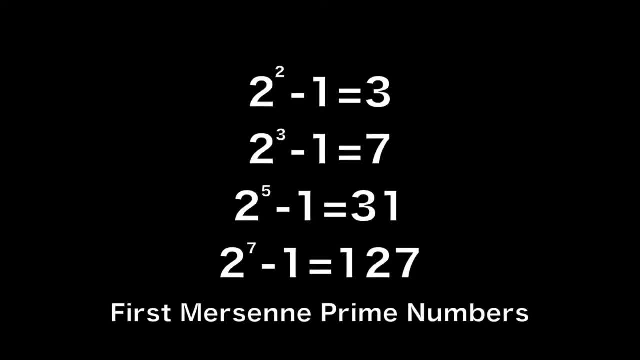 Two, three, five and seven. So the first four Mersenne prime numbers are two to the second minus one or three, two to the third minus one or seven, two to the fifth minus one or 31,, and two to the seventh minus one or 127.. Although there is a contest called. 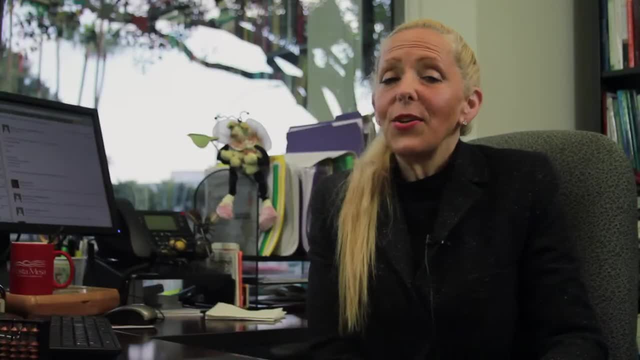 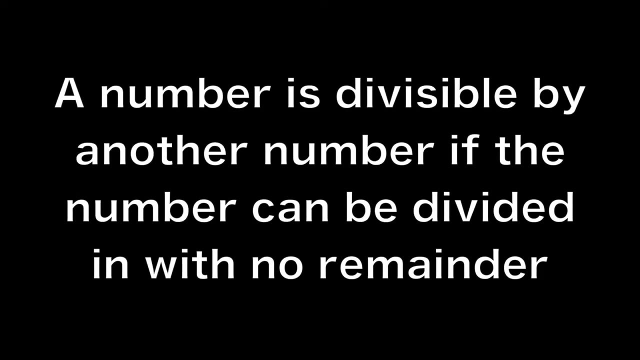 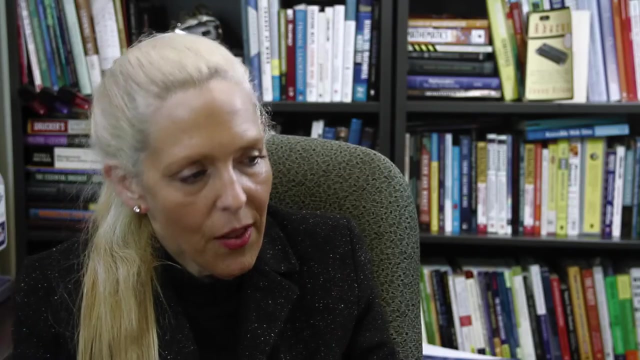 the Great Internet, Mersenne, Prime Search, any new ones found are determined digitally. Now let's talk about divisibility. A number is divisible by another number if the number can be divided in with no remainder, In other words, when you divide a number by another. 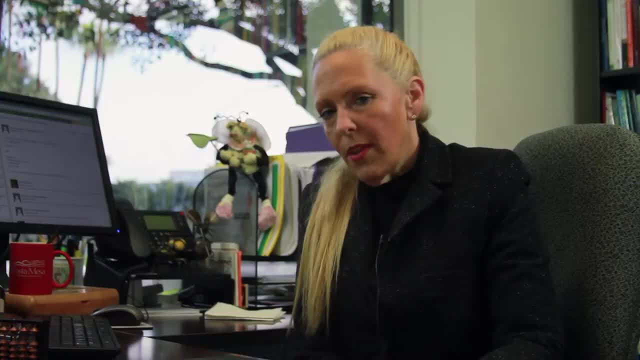 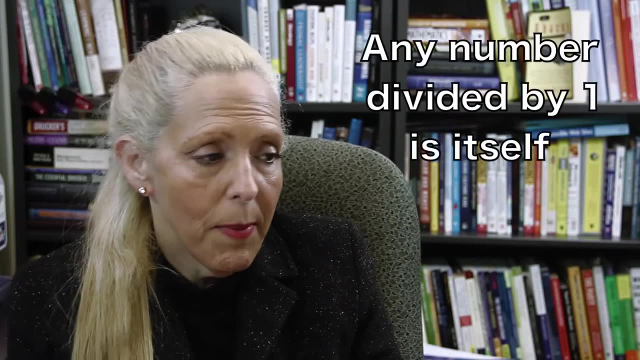 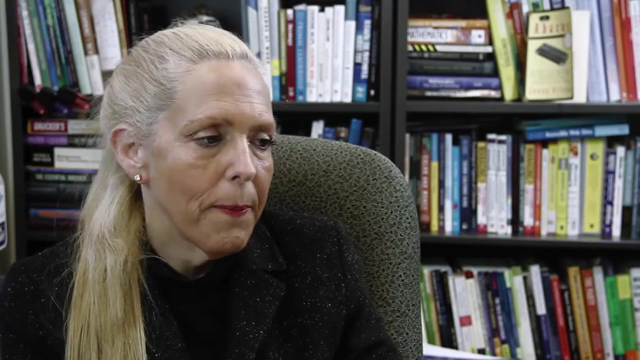 number, the result is a natural number. Remember that you can never divide by zero. However, you can divide a number by one. Any number divided by one is itself. So five divided by one is five. 143 divided by one is 143.. If a number divides into another number, it. 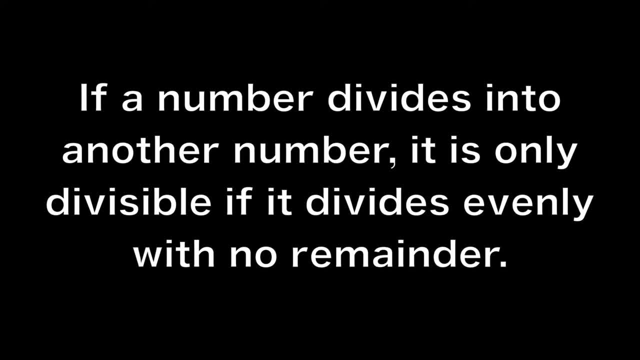 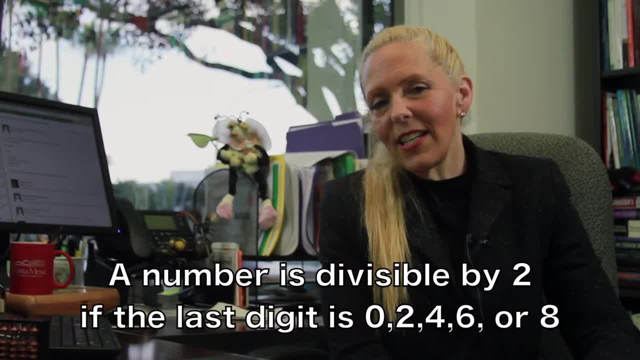 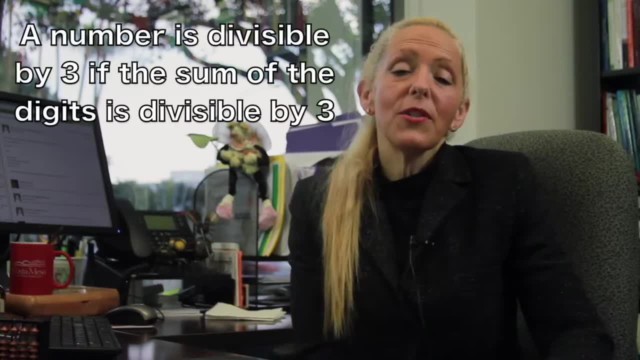 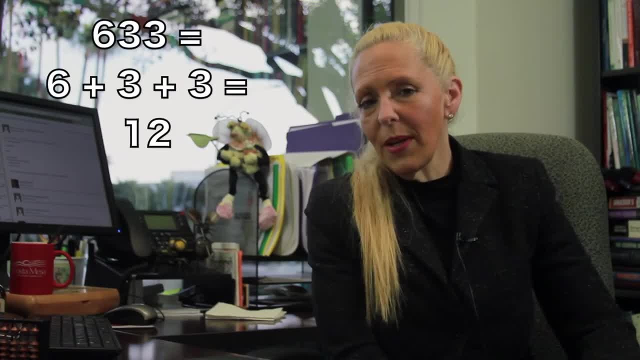 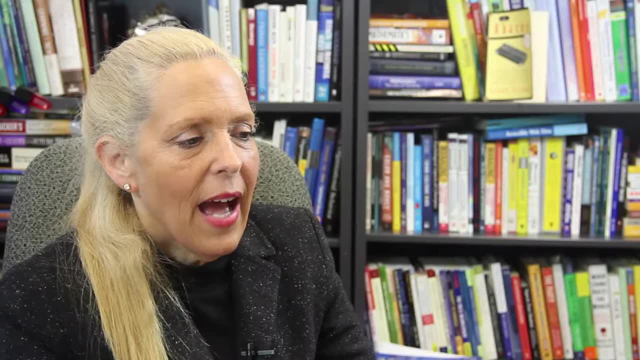 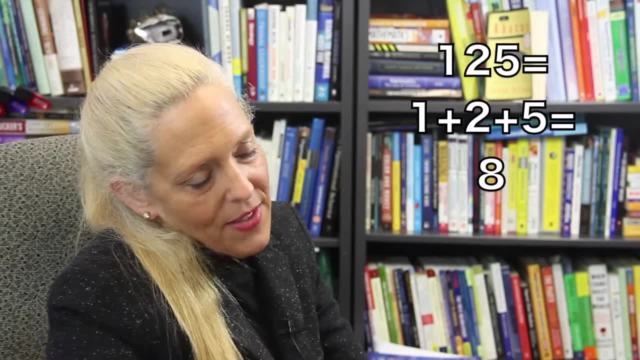 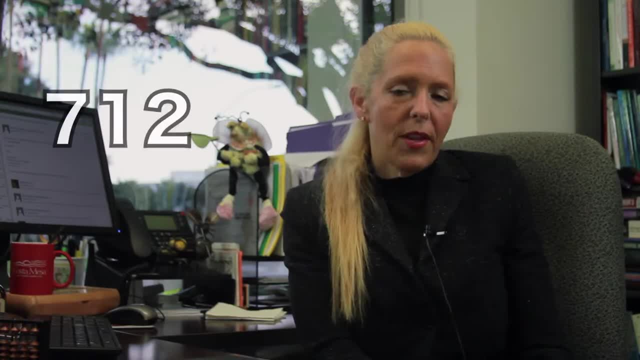 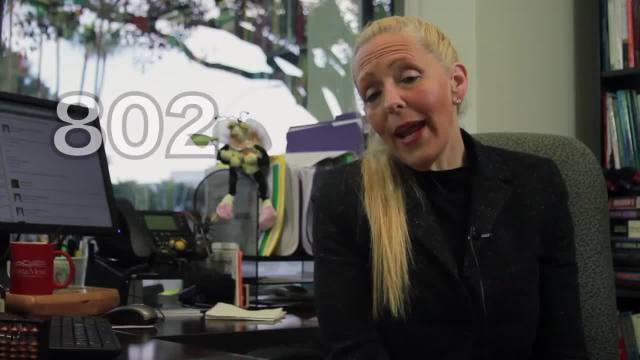 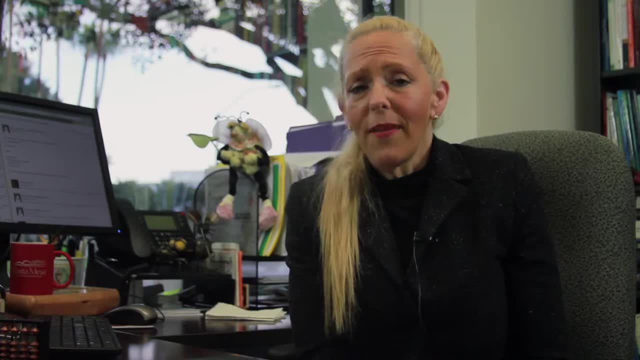 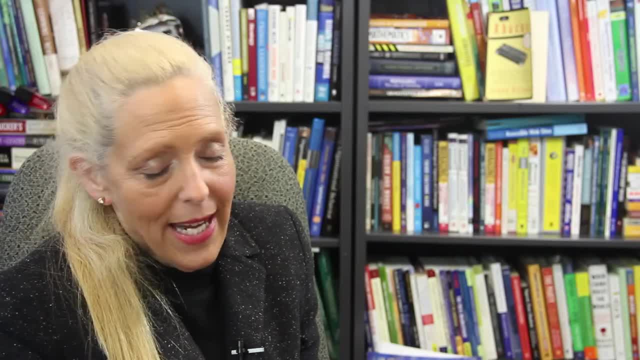 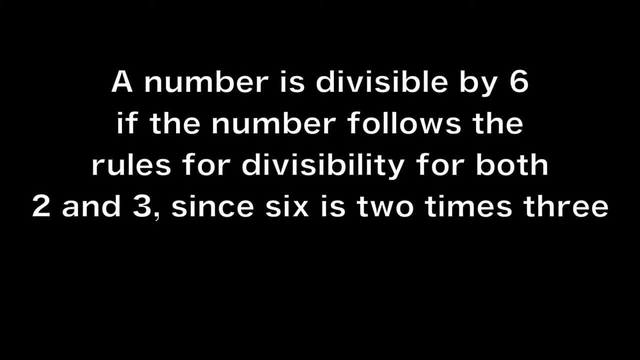 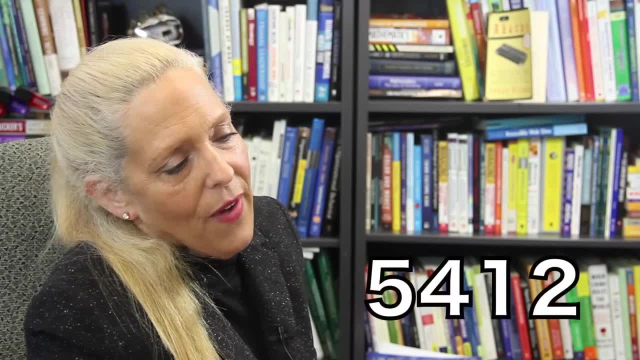 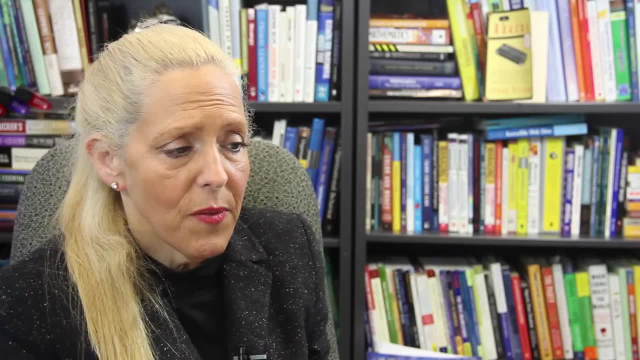 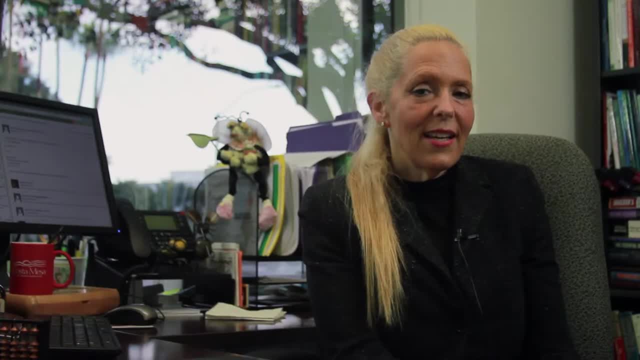 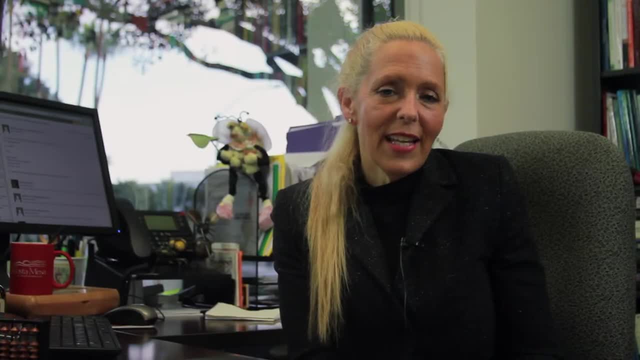 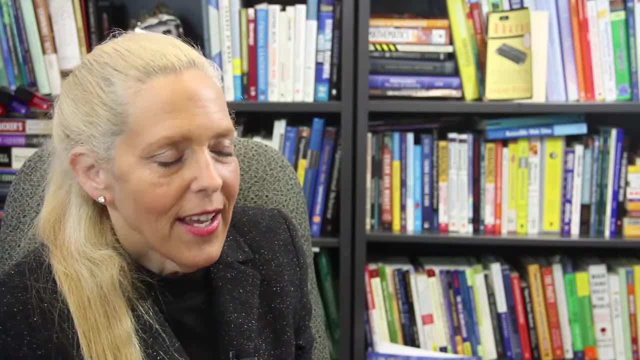 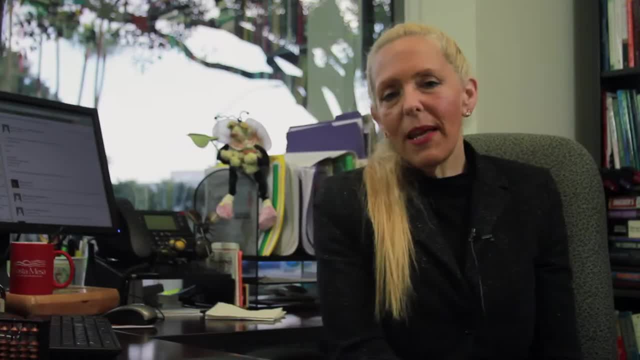 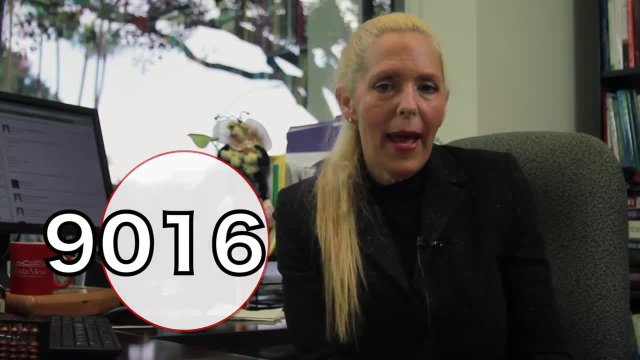 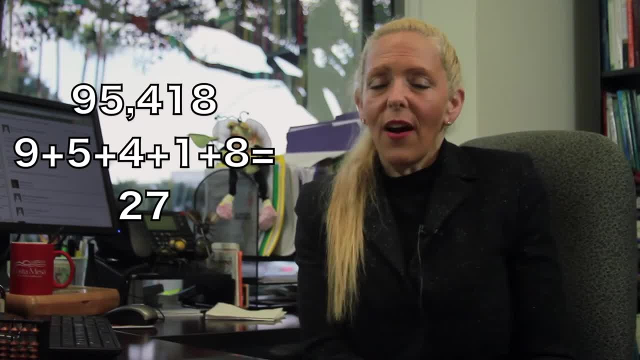 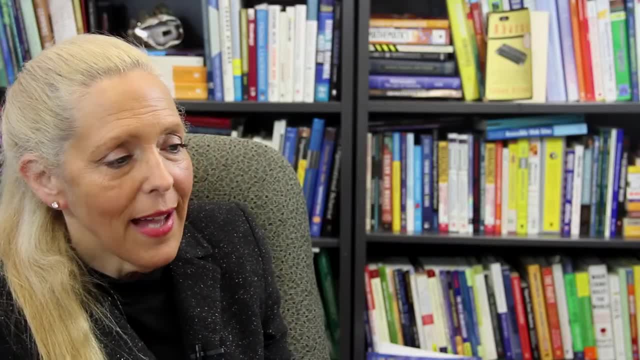 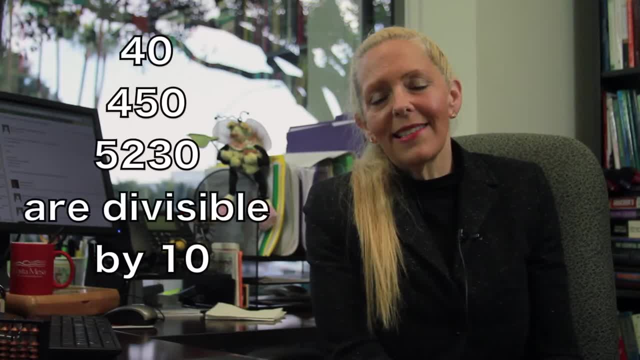 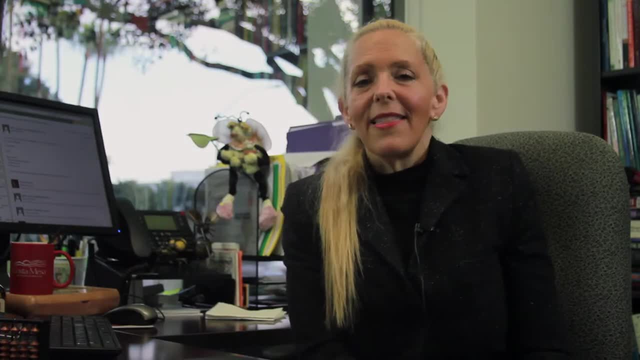 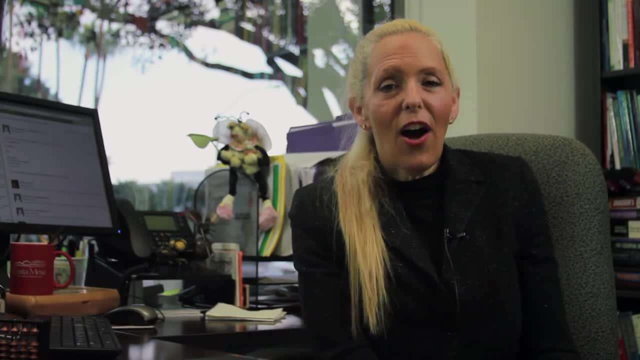 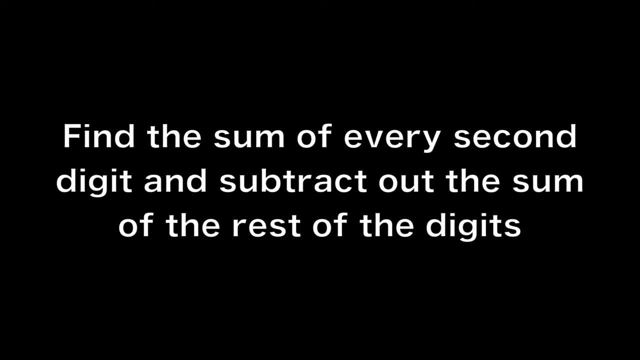 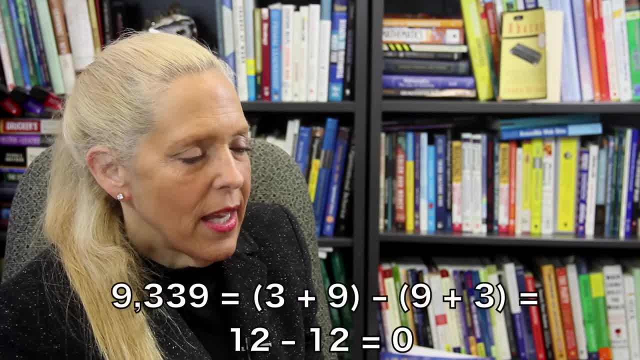 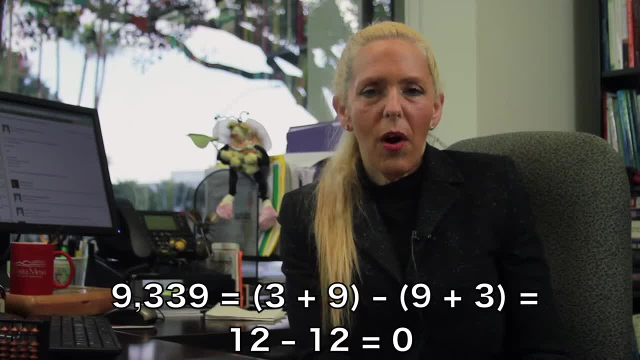 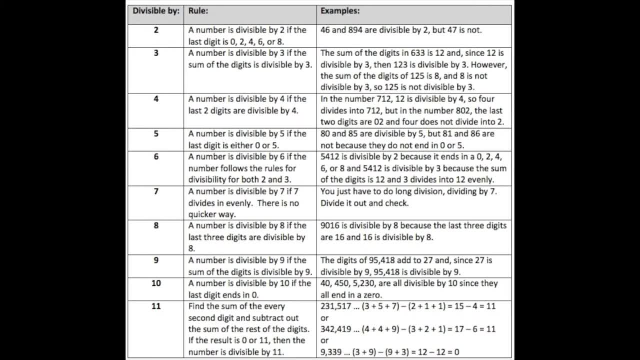 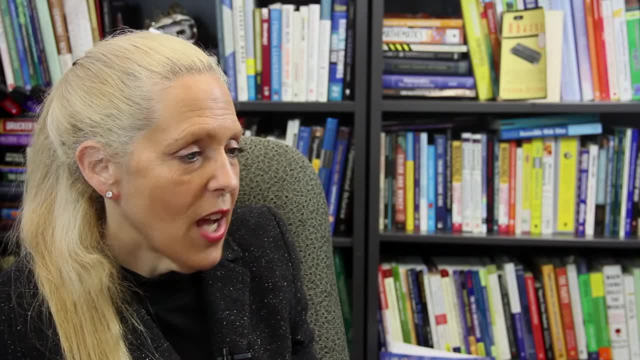 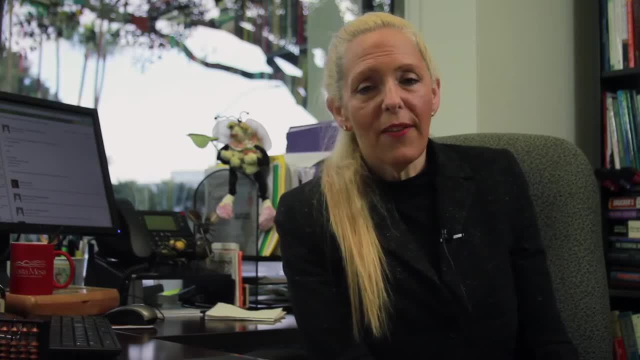 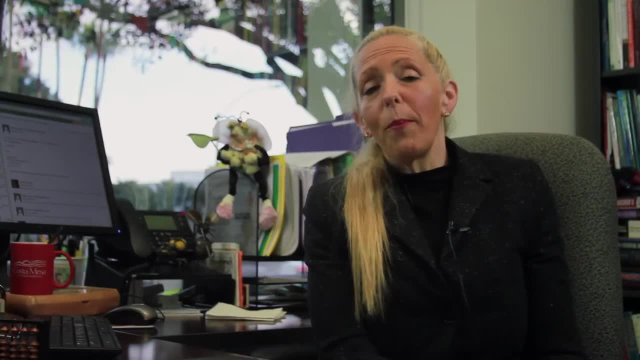 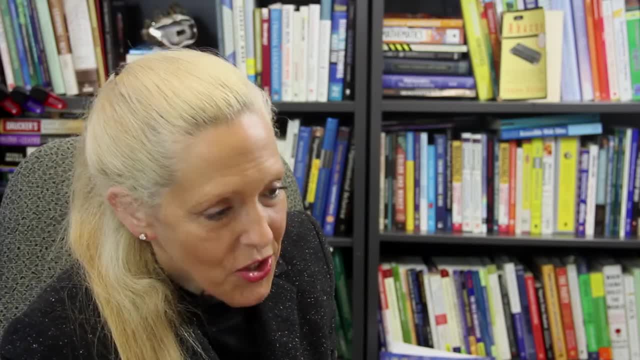 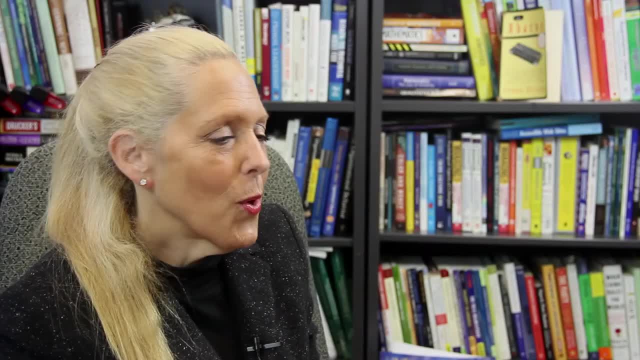 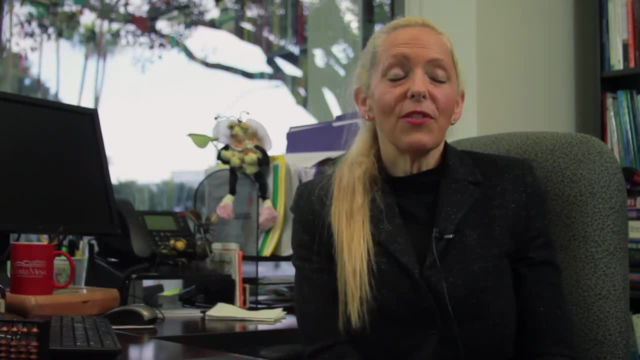 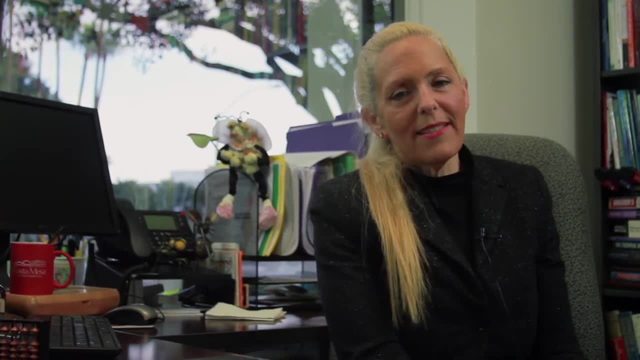 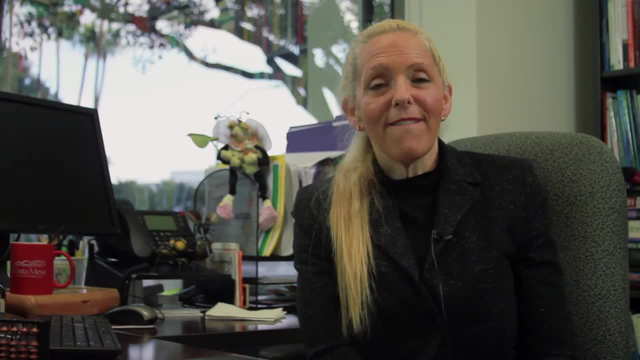